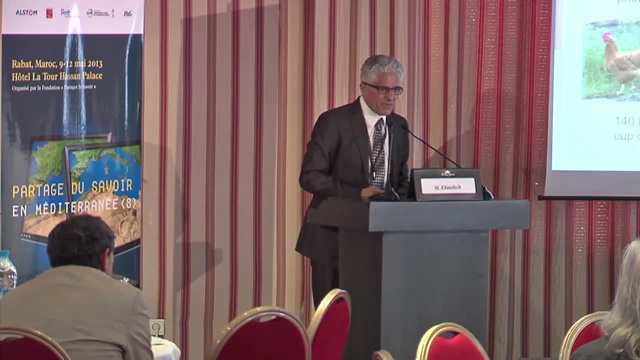 is the new oil. So now, when you think about water, each of us consume millions of liters of water, but you never think about it, because this is what we call virtual water. for each apple that you eat, each apple, you need to use 70 liter of water to get this apple. If you take one chicken, as you see here, you will have a 4000 liter just to have one chicken, And again in the US they'll have 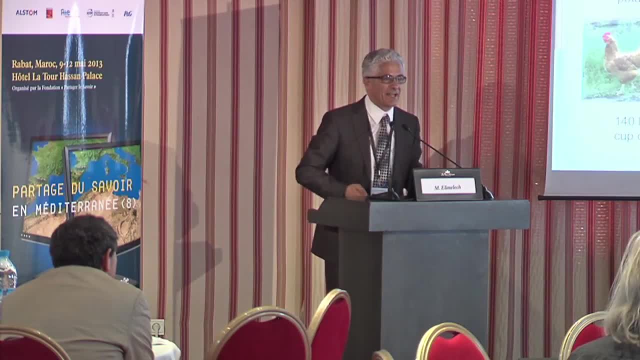 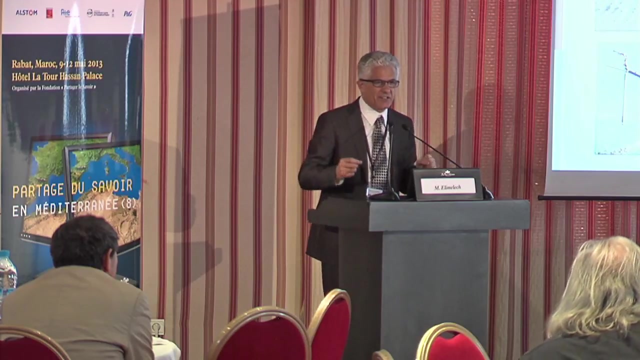 like a lot of hamburgers. It's 2004 liter for one double hamburger. It can be even worse if you have your leather shoes, and leather shoes can consume up to 17000 liter per kilogram of leather. So it's a lot of water that we never think about it, but it's, it's there. It's not just the water that you drink. Now I would say that also related to this water, energy, food, nexus. agriculture is really is a major, major consumer of water and we usually neglect it. We always think 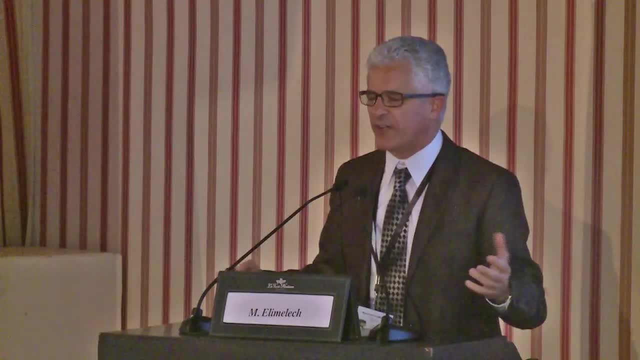 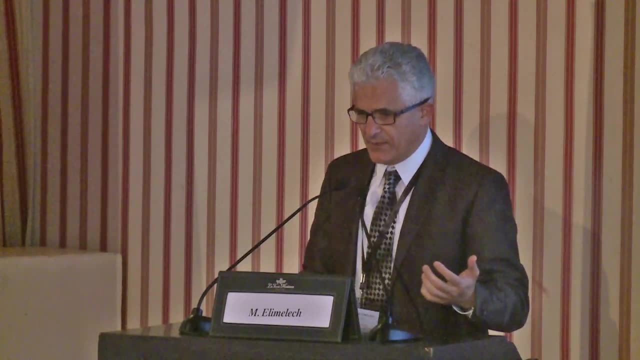 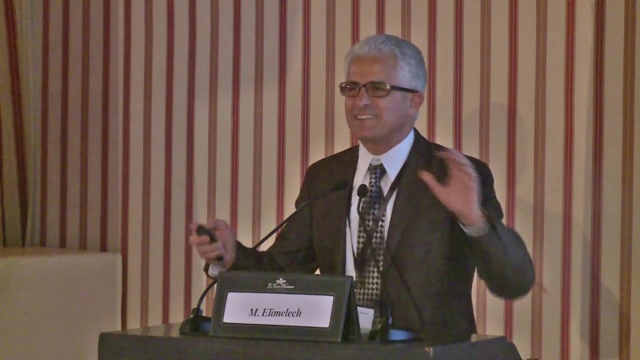 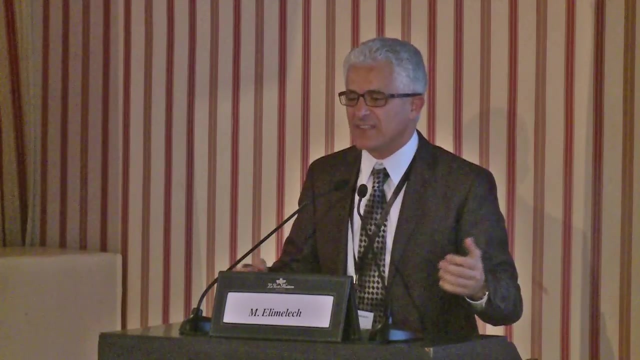 about industry and consumption and safe water, but agriculture is really the main driver of many, many water projects all around the world. So this is part of the conversion from a PC to a Macintosh, So we will suppose to have a nice diagram there to show the percentage of water for agriculture compared to other users and, as time, 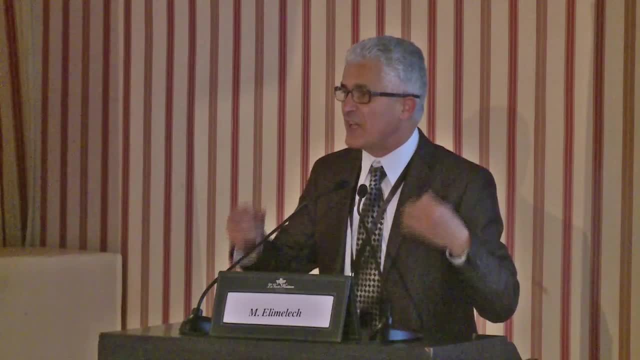 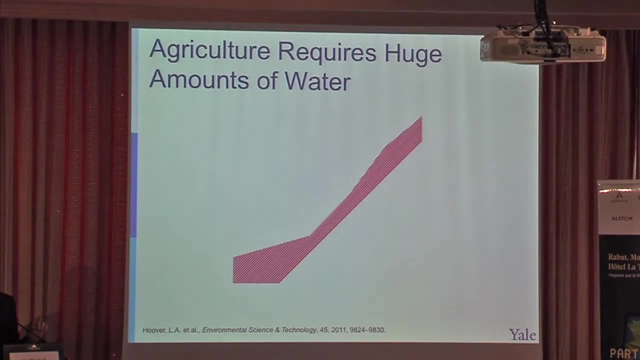 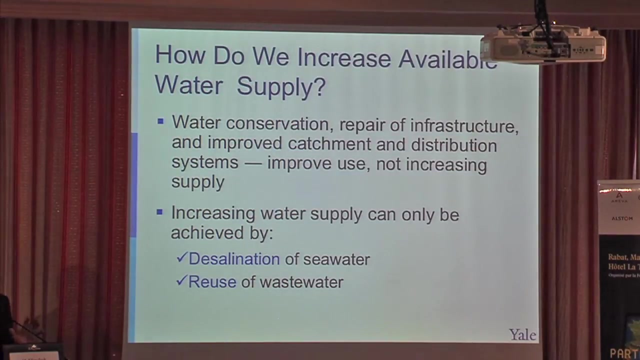 progressed. it's roughly about 70 percent. so 70 percent of the average water consumption is for agriculture. I hope my other beautiful slides will not be damaged. OK, we'll see some other, But conversion from PC to Macintosh: We need to have something more. some of the technologies. 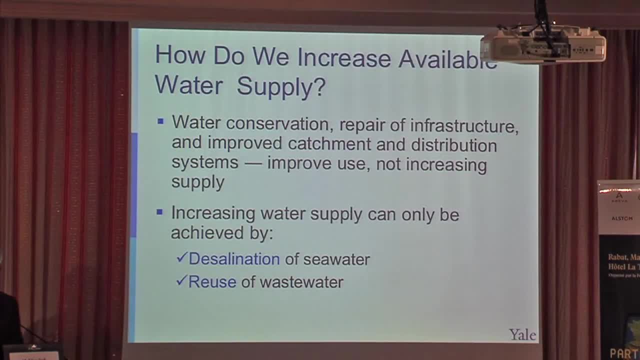 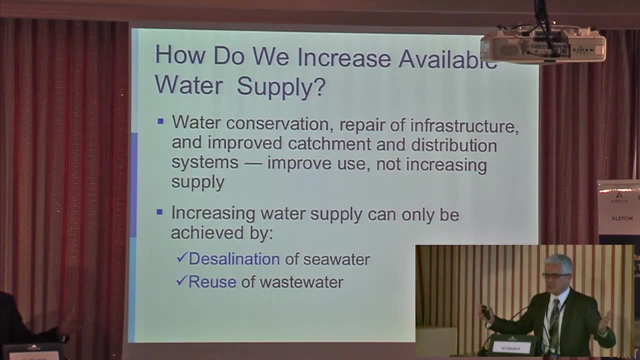 here to find some way to- Or maybe we all should convert to Macintosh. I'm sure Robert will like it. So at least now I convince you, or at least I tell you that there is not enough water. So the question is: how do we increase? 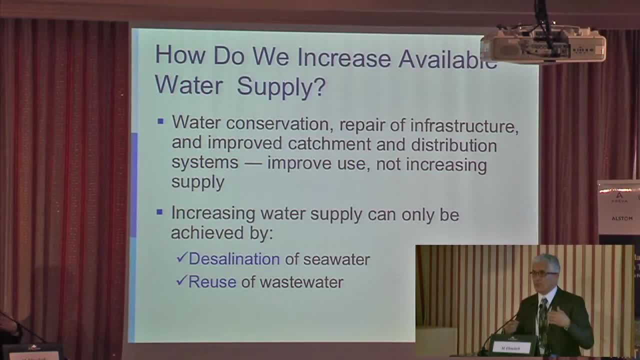 the available water supply. So of course, we can do all the usual things that we always were told We can do- water conservation, repair of infrastructure, improve catchment- But all of these will improve the use of water And they will not give you more water. than what you can get from the hydrological cycle. The only way to get more water than what you can get from the hydrological cycle is to turn to engineering And either desalinate seawater- We have plenty of seawater- Or recycle all the wastewater. 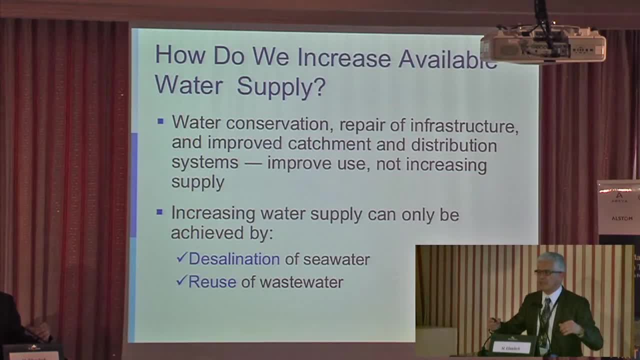 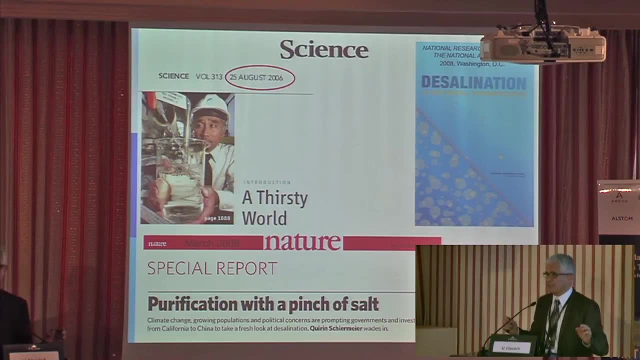 And it's done in many, many countries- Singapore, US, Israel- they recycle all their wastewater And they use a lot of desalination. So I will focus only on desalination and talk about some of the technologies. Now, desalination also got a lot of coverage. 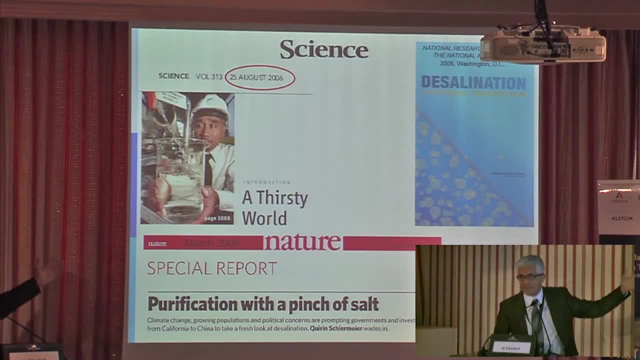 by even high-profile magazines like Science and Nature, the dedicated special issue that talk about water And desalination, And the US National Academies also wrote a big report about desalination, asking if it really can be a solution to global water scarcity. 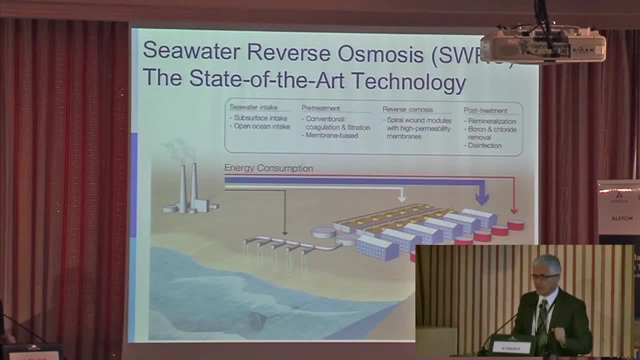 The main technology nowadays for desalination is reverse osmosis. This is the predominant technology for all the new desalination plant, except someplace in the Gulf country that they have still the thermal desalination, which are more energy intensive. 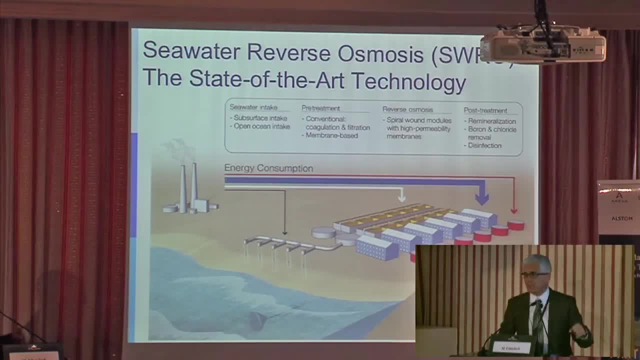 It starts with the intake of water from the sea, goes through some pretreatment that in principle similar to the way we treat water for drinking water. Then it goes to reverse osmosis. that does all the separation of water and salt. This is most of the energy. 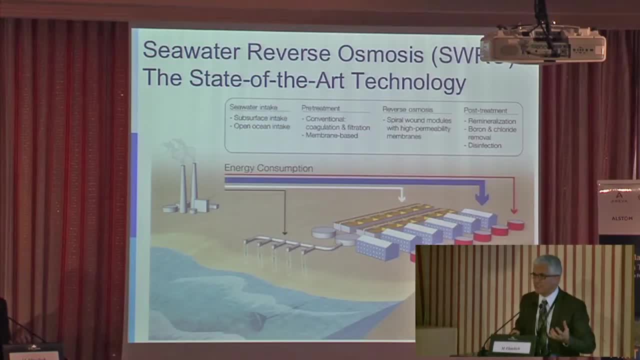 As you see, from the thickness of the line, most of the electricity comes for this process, And then you have post-treatment to remineralize, And also, when you talk about agriculture, the post-treatment that is very, very important is to remove. 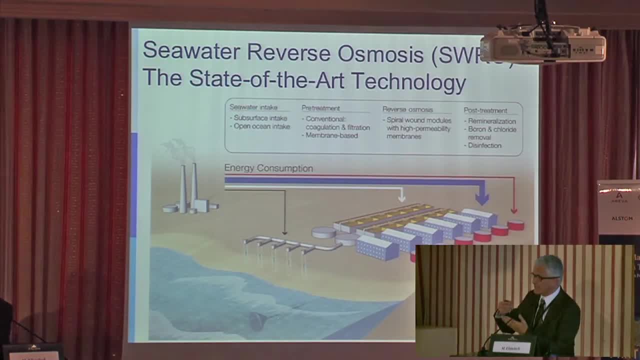 boron and some chloride, Because boron is not rejected well by these membranes And if you have high level of boron it's not good for many, many crops in agriculture. So boron and chloride need to be removed And this can be quite costly. also the extra polishing. 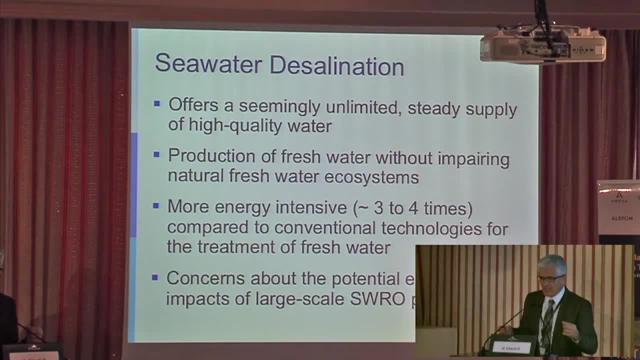 So just a few words about desalination before getting in-depth. It offers seemingly unlimited steady supplies of water. The ocean is vast, You'll have it all the time. Now also, it can produce water. It can produce water without impairing. 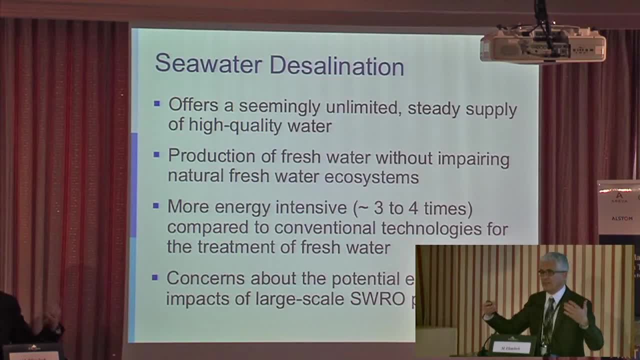 the natural ecosystem. If you take waters from river and lakes, you can affect the ecosystem. You need water from the ecosystem, The ocean. whatever you take, it will be just like one drop. It's insignificant. However, and this is what I will emphasize- 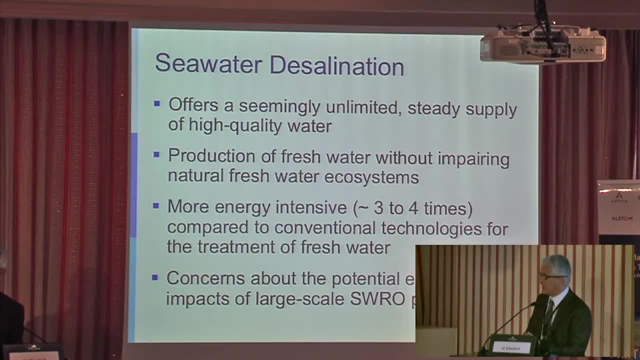 it's much more energy intensive. It takes about three to four times more energy to desalinate than the way you treat water, For example, the water that is treated from the river in Rabat and come to your tap water. It's about three to four times more energy. 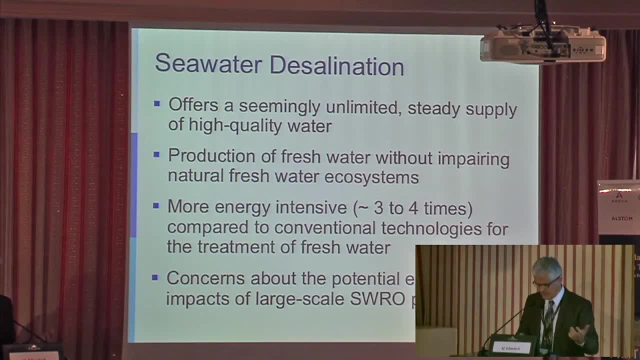 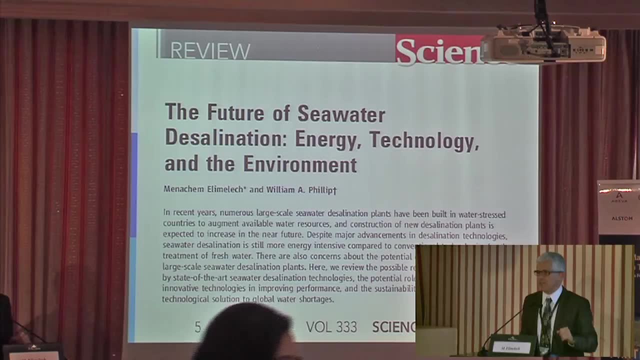 And there are some environmental concerns about desalination. So I wrote a review article about a year ago that covered some aspect of the seawater desalination And here I will highlight only a few things and add some more of the newer things. 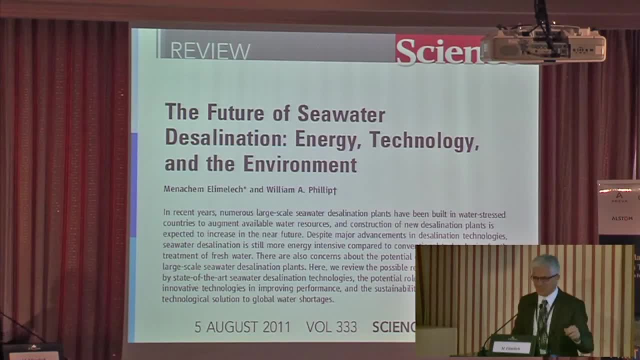 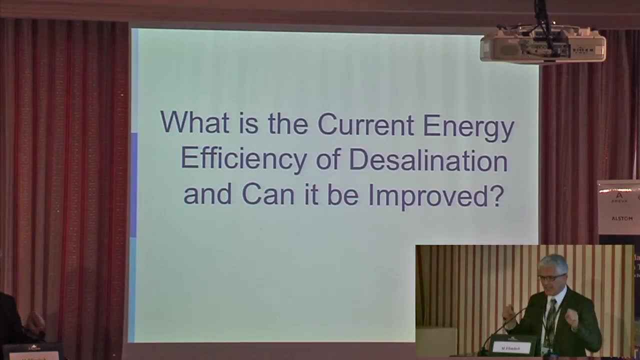 And I know Robert told me that he read this article just before I came here. So I would like now to pose two main questions: What is the current energy efficiency of desalination And how can it improve? Because we really need to understand. 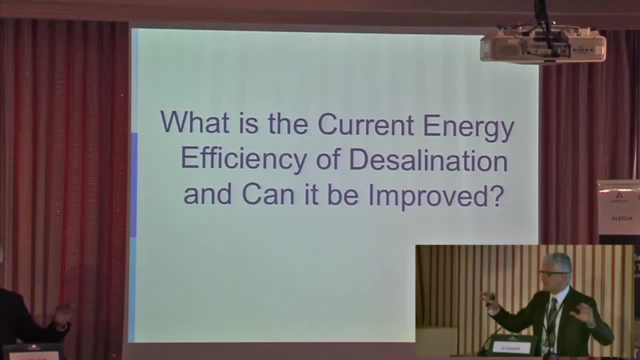 what's the limit, or thermodynamic limit, of desalination? Because someone can come to you and tell you: I can do desalination with I don't know 0.1 kilowatt hour per cubic meter, and you will believe him or her. 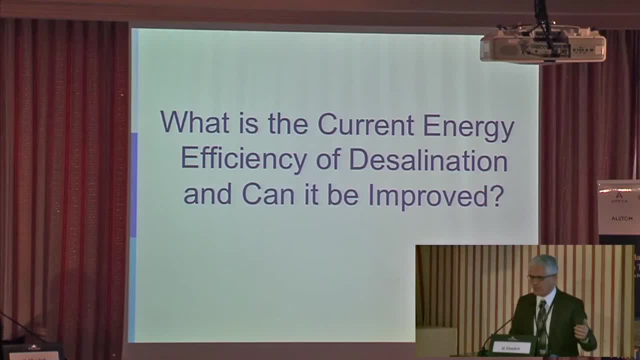 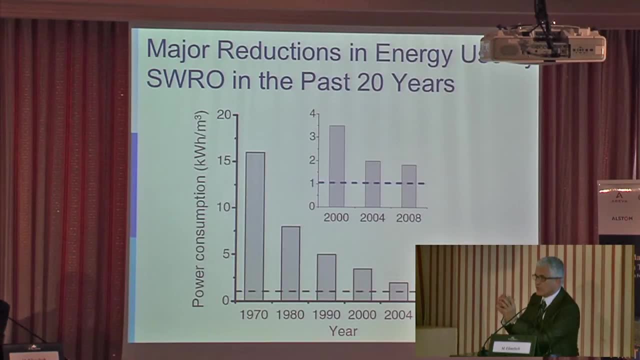 It's not the case. There is some limit that you cannot violate, and it's based on thermodynamics. So I would like to show you a diagram of the energy consumption just by the reverse osmosis stage, the one that takes the separate water and salt. 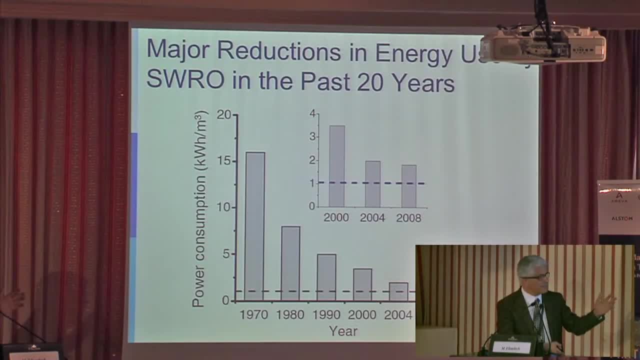 Since the reverse osmosis was invented in the late 60s until now, And, as you see, the energy consumption achieved a plateau. Now this was a paper that we have written, but in principle, if you go now, it's about the same. 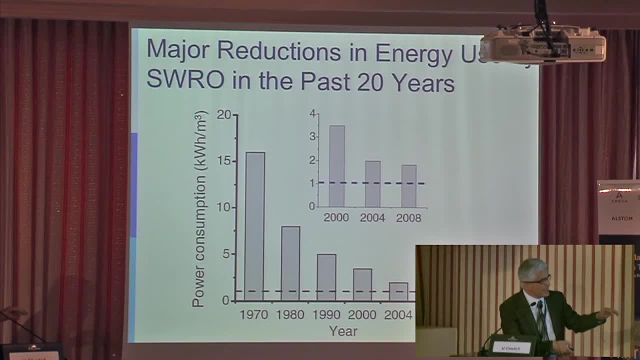 It doesn't change, And note this line. I will describe more the dashed line that you see here. This is the thermodynamic limit that I'm going to describe very soon. Most of the improvements were done here due to a better system, some better energy recovery system. 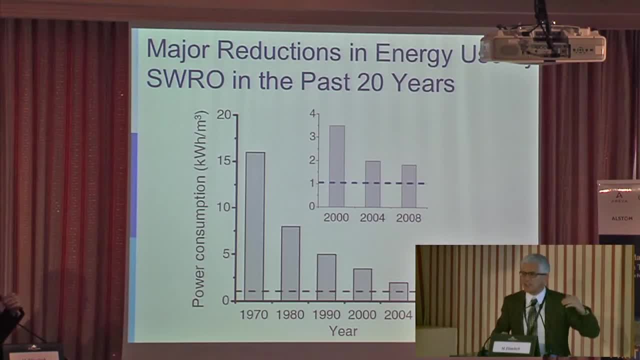 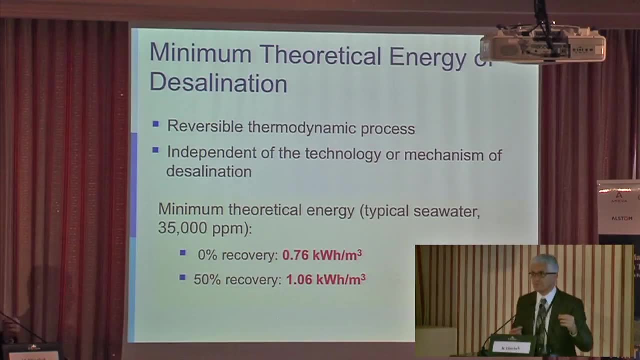 and better membranes, But you reach now a limit that you cannot improve farther, and you are very close to what we call the thermodynamic limit of desalination. So this is what I would like to say, a few words From thermodynamic. you can calculate. 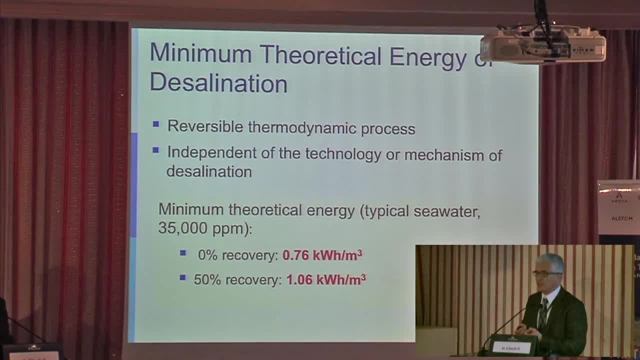 how much energy required to separate water from salt, And you cannot do it with less energy. This is what thermodynamic dictates. This is the limit. So if you take seawater- 35,000 ppm and you take just one drop of water from the seawater, 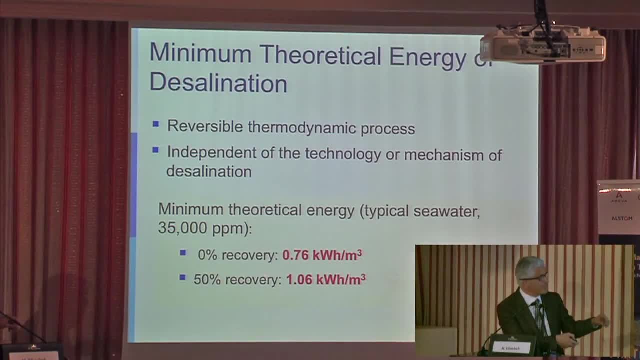 you will need 0.76 kilowatt hour per cubic meter. Now most desalination plants work at 50% recovery. It means for each volume of water you will get half clean water and half become concentrated. For this thermodynamics tell you you cannot do it less. 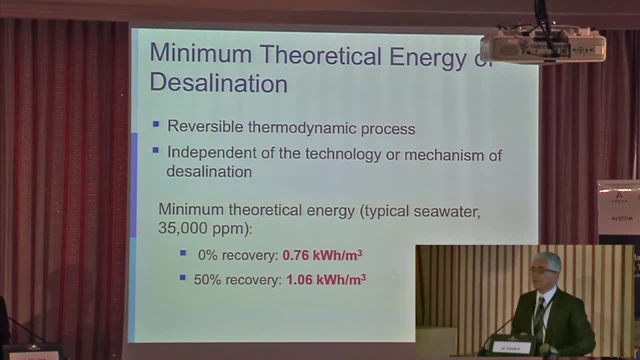 than about 1.1 kilowatt hour per cubic meter. It's impossible, even if you invent the most, You just cannot. And it's independent of the process. It's just based on thermodynamics. So you can't do it with less energy. 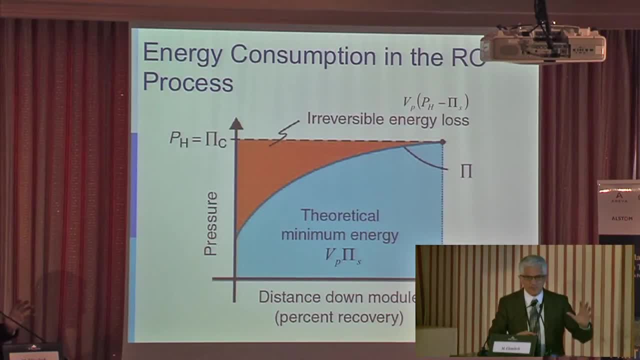 Now, desalination plants require more And because I will explain it just briefly, In principle, the way you desalinate, you have membrane modules, like a channel with membranes, And you can think about it that the seawater starts here. 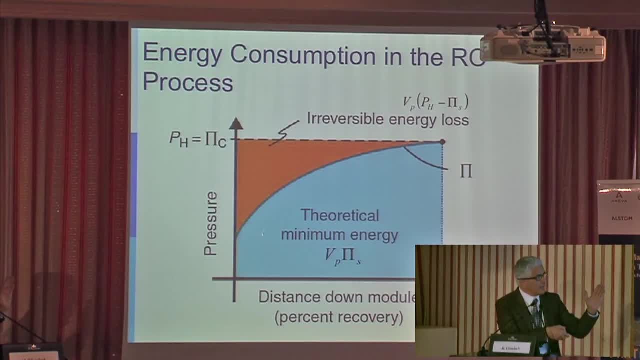 And the seawater has some kind of osmotic pressure, maybe 27 bar, And as the water coming through the membrane you squeeze fresh water, the salt inside these membrane element increases And when you exit the modules usually it's about 6 meters long. 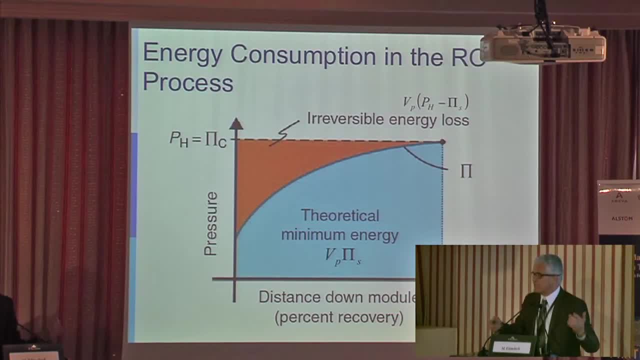 It becomes much more concentrated. So, for example, if you start with seawater of 35,000 ppm, 25 bar, at the end of the membrane you will have 50 bar. So you cannot operate the reverse osmosis with less pressure than this osmotic pressure of the exit. 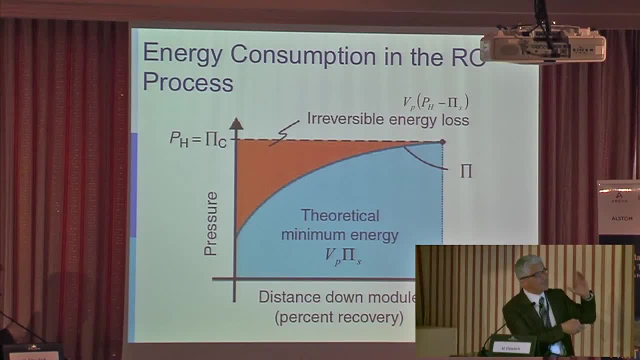 So you must apply this pressure, Otherwise you will not get water coming out from the membrane of some part here. Remember this part because we will talk about it when we talk how much we can improve desalination. In reality you apply a little more pressure. 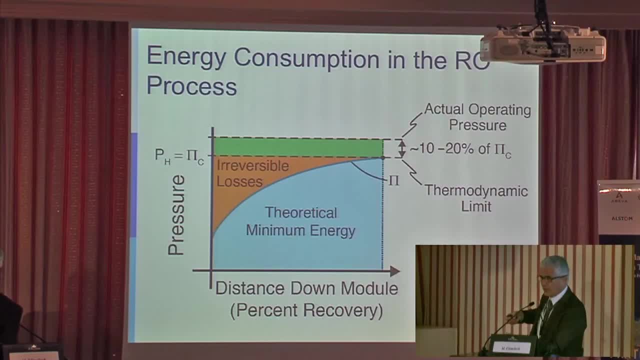 because of the frictional drag as water flow in the channel, There's some friction and energy losses. so about 10%, 20%. So this is the way you can operate. If you operate at less pressure, you will not be able to squeeze water. 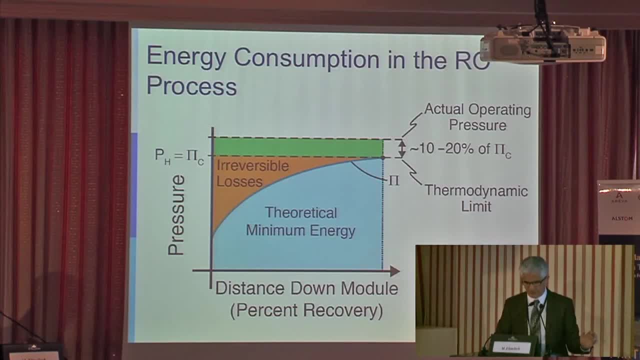 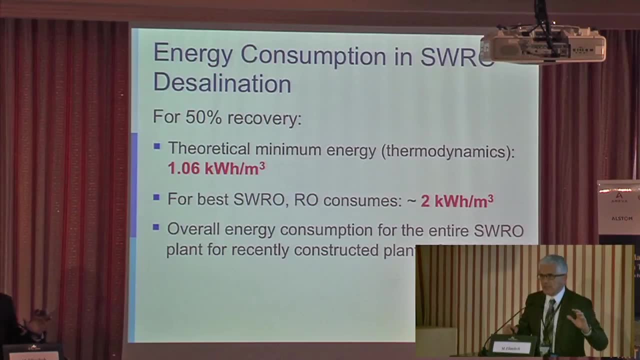 through some areas of the membrane. So remember this part Now. so just summarize the values. So the minimum energy by the reverse osmosis is about 1.1.. The best desalination plant that is built nowadays, like the one in Singapore, Spain and Israel. 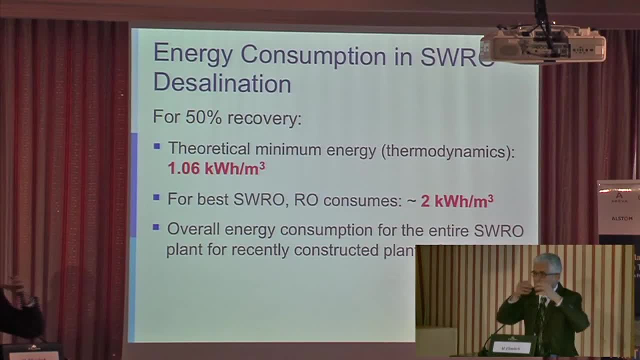 they do it around 2 kilowatt hour per cubic meter just for the reverse osmosis stage. However, when you look at the entire consumption of energy by the entire desalination plant, remember there is pre-treatment and post-treatment. is about 3 to 4 kilowatt hour per cubic meter. So again the output is about 1.1.. RO, just the reverse osmosis, consume 2 kilowatt hour per cubic meter. The rest of the plant is about 3 to 4.. 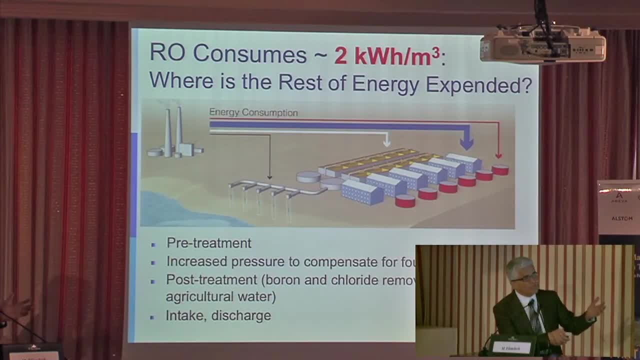 And the rest of the energy comes from the intake, the pre-treatment and many times the post-treatment. To remove the boron after the desalination stage sometimes you need to have another reverse osmosis or even two reverse osmosis stages. 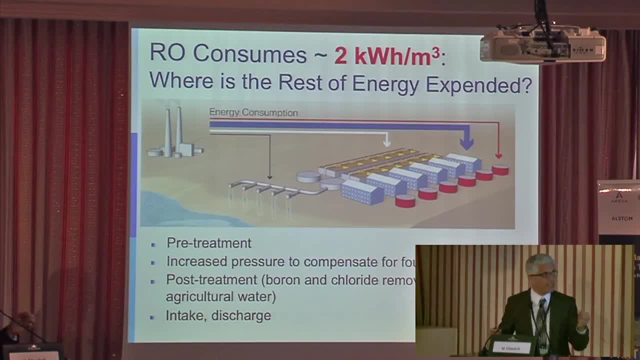 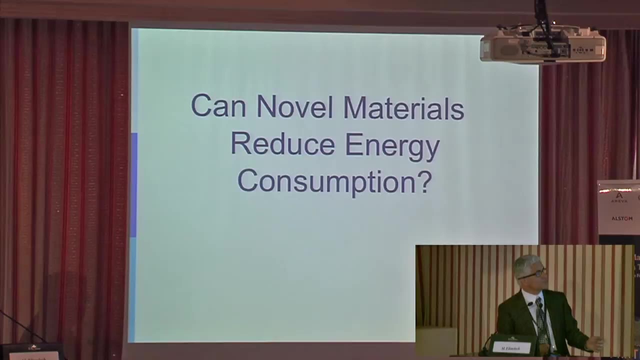 And otherwise you cannot use the water for agriculture, And this is very important. Desalination becomes a source for water for agriculture, Like in Spain. I heard now in Agadir, Morocco, they build desalination plants for agriculture, And the same way in Israel they use it for agriculture. 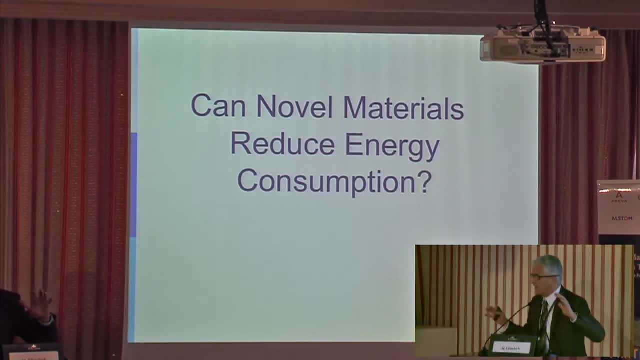 So now that we know roughly the energy limit of desalination, let's see how we can improve it. So there was a lot of research that said that if you can get better materials, we can make desalination much more energy efficient. 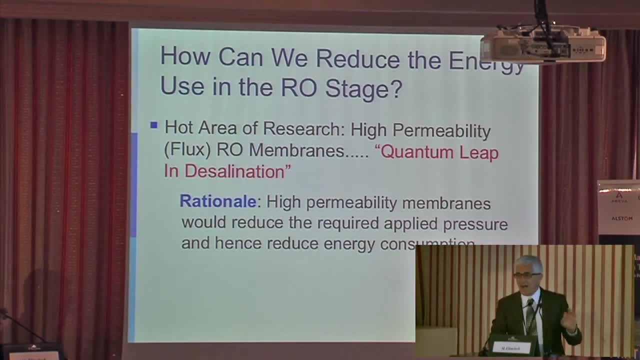 And I would like to tackle this problem. One of the hot areas of research until recently was what we call high permeability membrane. They promised: if you make this membrane with the high permeability, which means the water will go there almost with no resistance- 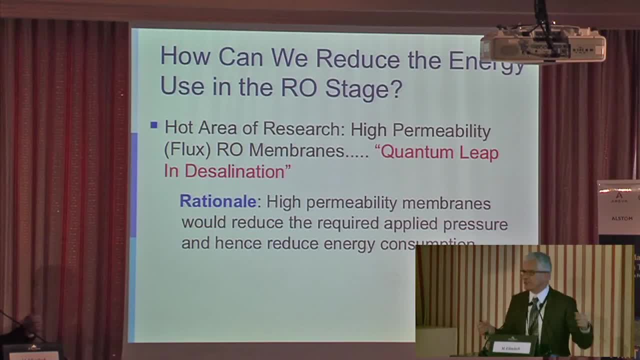 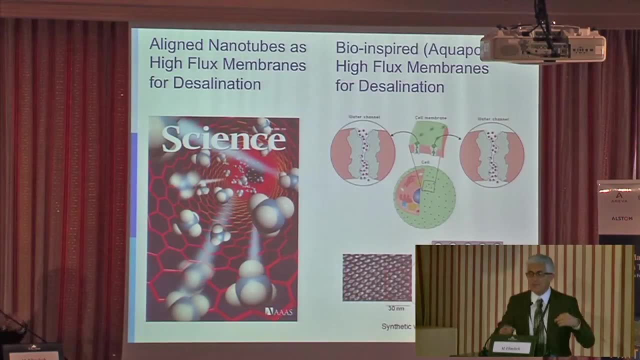 you will have a quantum leap in desalination. You will save a lot of energy and desalination will be as cheap as making water for treating the river water. And some of the areas of research that they got into are two. One of them is aligned carbon nanotube membrane. 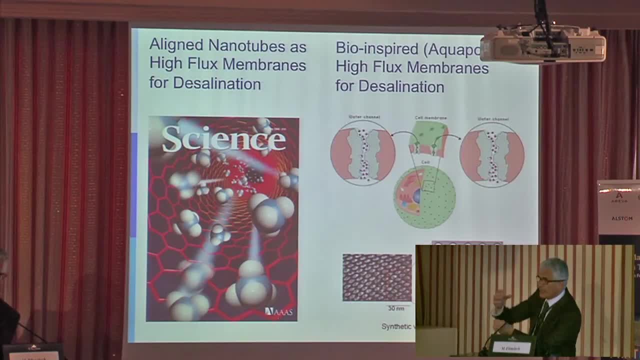 They found through simulation that it's a very high permeability membrane. They found that if the water goes through this carbon nanotube, there is no friction because the carbon nanotube are smooth and hydrophobic and the water goes with no friction. 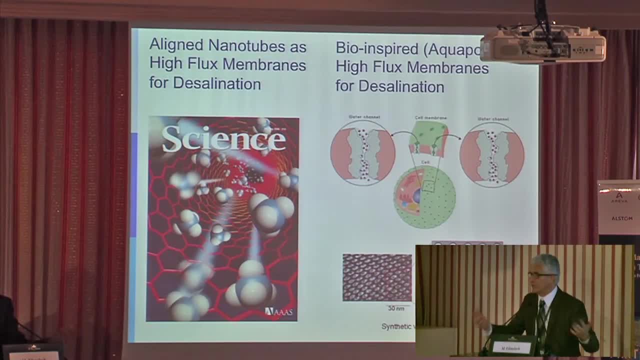 You can get very, very high permeability And they said that if you use it in desalination you will have almost no energy. The same thing with some of the biologists here. Aquaporin- this water channel- are known to pass water at very high flow rate. 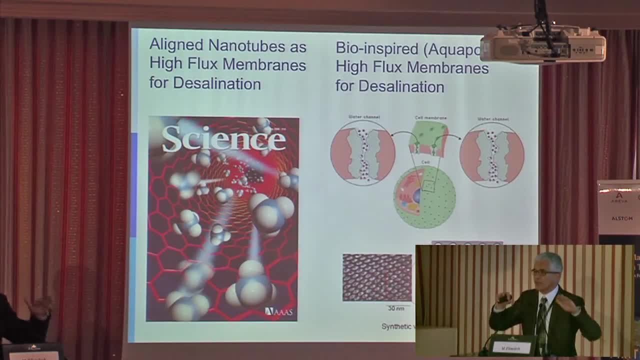 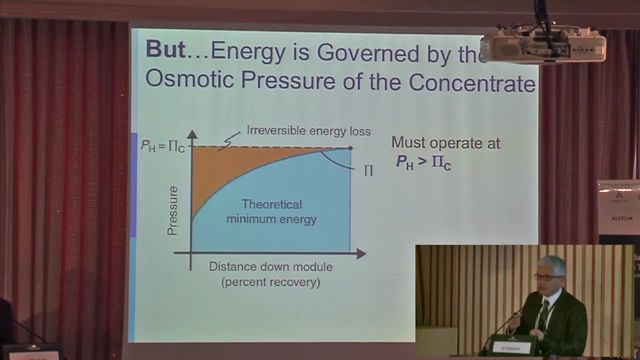 And they suggested to incorporate them into membranes so that they can reduce the energy of desalination. But I would argue that it's not the case, because the flow or the transport of water through the membrane is governed by the thermodynamics, not by the resistance of the membrane. 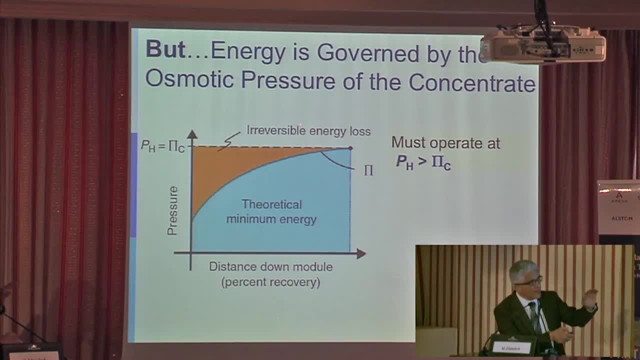 because of what I explained to you here. You must operate with at least this pressure to get any water coming out because of the osmotic pressure of the brine as it accumulates in the membrane channels, And you need also about 10%- 20% more to compensate. 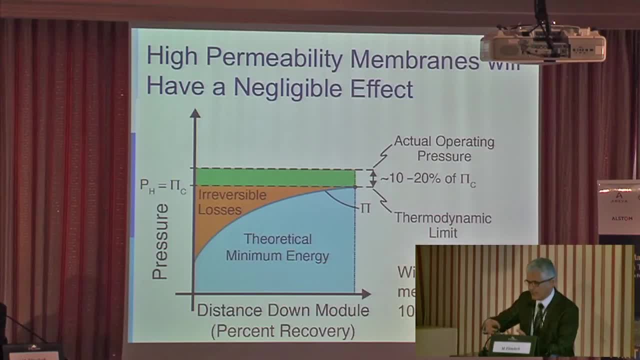 for the low concentration, polarization and frictional drag or pressure drop. And it just happened that the current membranes that we are using nowadays already operate just about this range here. So if you have high permeability membrane, you will not use less pressure And pressure. the energy is just proportional to the pressure. 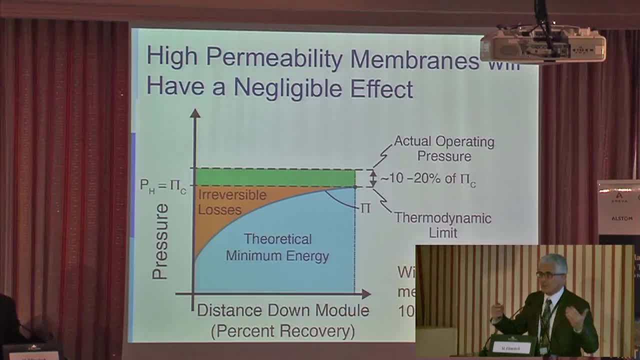 So you cannot use and desalinate with less of this pressure And the current membrane already there. So this high permeability membrane. even again, they're not even demonstrated. You can desalinate, but even if they would be there, 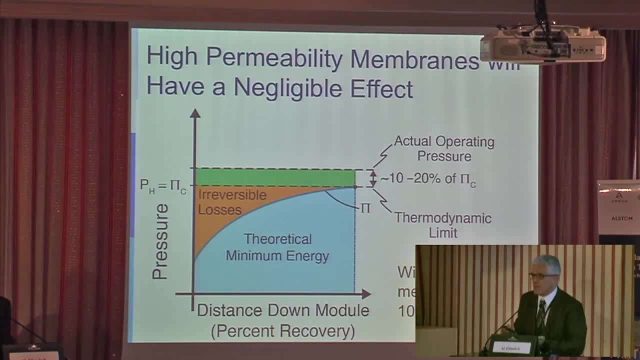 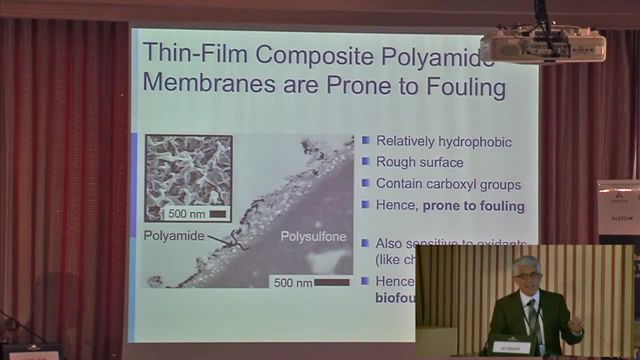 they maybe just reduce the area needed for desalination, the membrane area. But the membrane is only 5% of the total cost of the desalination, so it's not significant Now the state of the art in desalination. 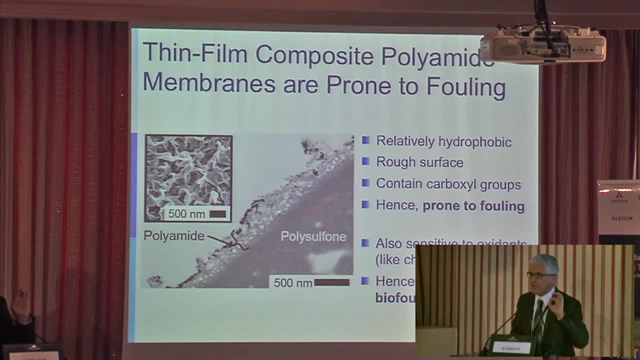 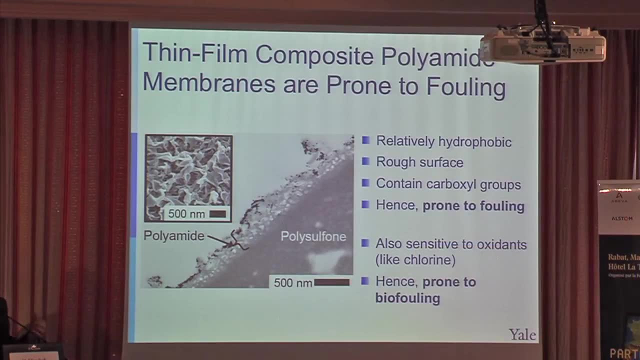 are these thin-film composite polyamide membrane. They are very permeable and selective. They retain 99.9% removal of the salt, so retain more of the salt and get very high water permeability. However, there are many properties. 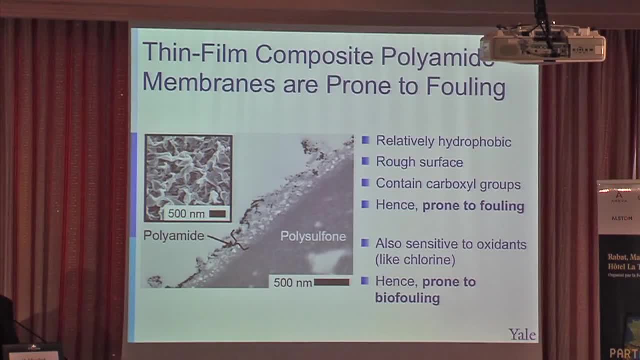 that make them prone to fouling, And fouling is the process when you have all these substances in the water that attach to the membrane and affect their performance, like organic matter particles that accumulate and foul the membrane so it becomes less permeable. 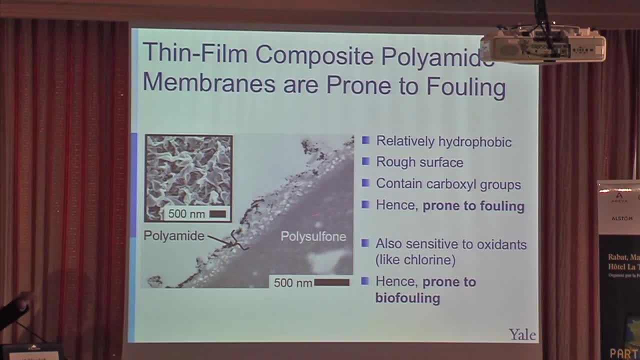 Because they are hydrophobic, they have rough surface, they contain carboxyl group and also they are sensitive to chlorine and oxidants. So many of the properties will make them so you will not be able to clean them effectively. They will foul. 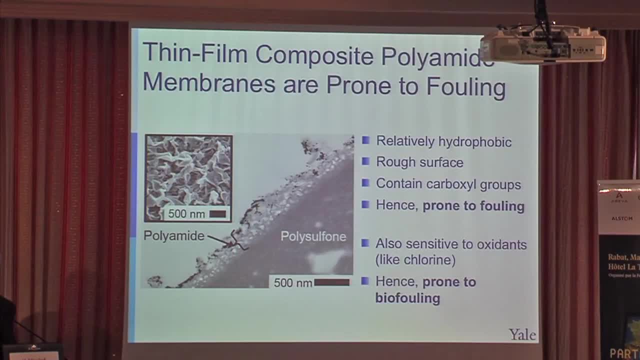 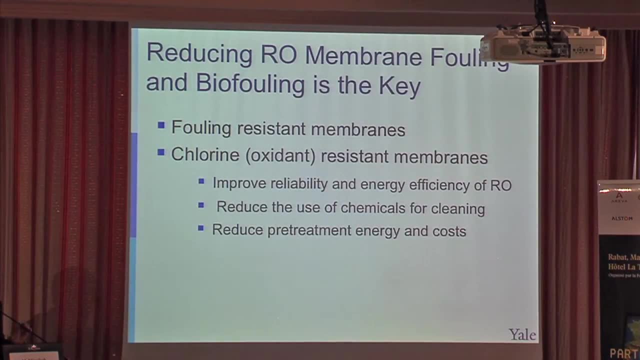 And once you have fouling of the membrane you need to increase the pressure so you can squeeze the amount of water that you want. So I would argue that really the improvement that the high permeability membrane will not improve the energy of desalination. 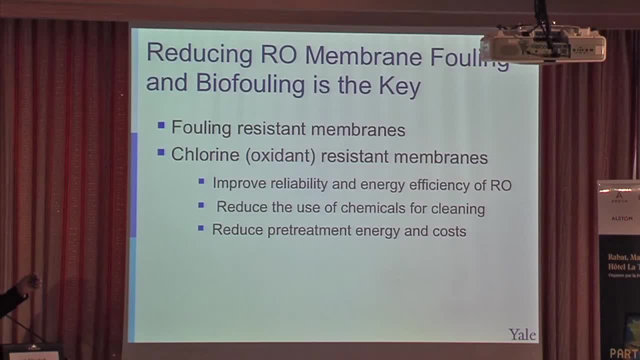 because of what I explained And what you really need is. the key is really to get fouling-resistant membrane, because the current membranes are prone to fouling And also membranes that can tolerate oxidants like chlorine. the current membrane, the polyamide membrane- 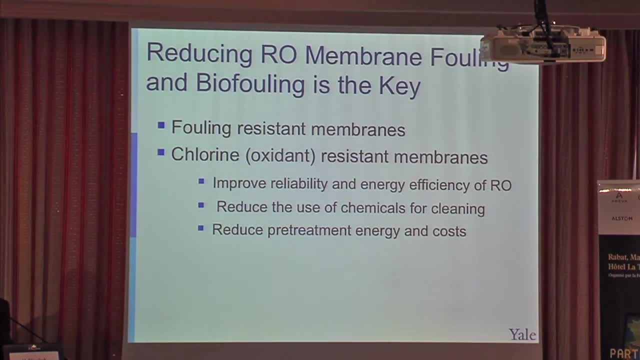 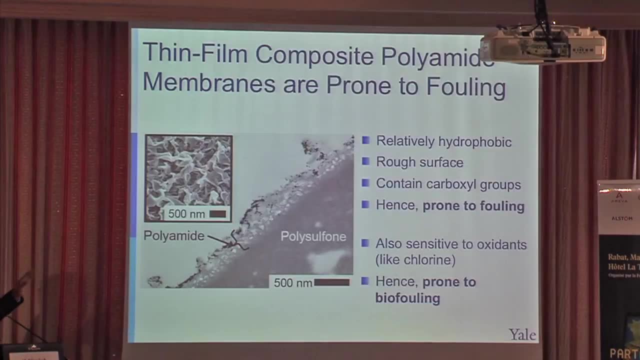 if you have chlorine, it will degrade and will not perform well. Now the membrane companies and scientists try for the last 30 years to find a better membrane than this polyamide chemistry, and they cannot come up to something. Whenever you come, something that gives you a little more flux. 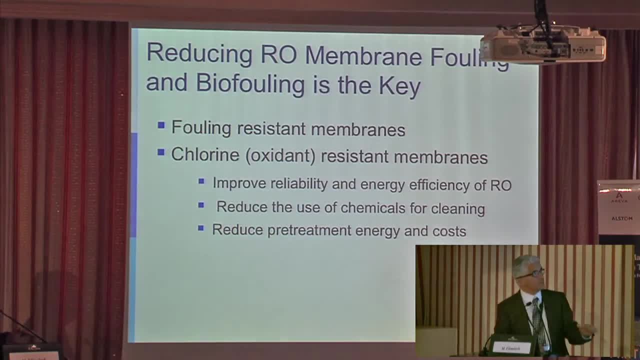 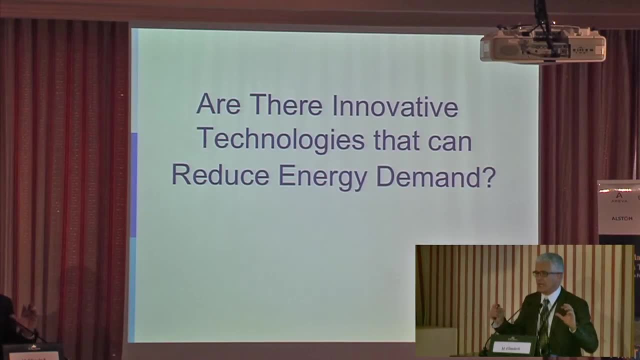 then it cannot reject a lot of salt. So the future I mean is really in these materials are to make fouling-resistant membrane and all these nanotype membranes, And if you have a very high permeability membrane then you can't do anything about it. 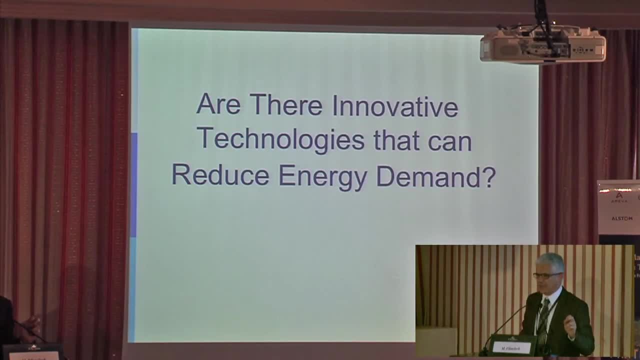 So I would argue that the high permeability membrane will not reduce the energy of desalination. Now here again. my original topic title was forward osmosis desalination. And the second question that I pose: are there any technologies that can reduce the energy demand? 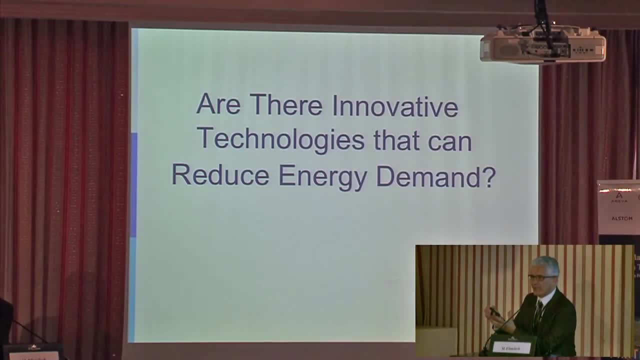 I talked only about the reverse osmosis technology. The other technology that's used in the Gulf countries is thermal desalination, That you practically boil the water and it's not energy intensive. So they will never be able to compete with desalination. 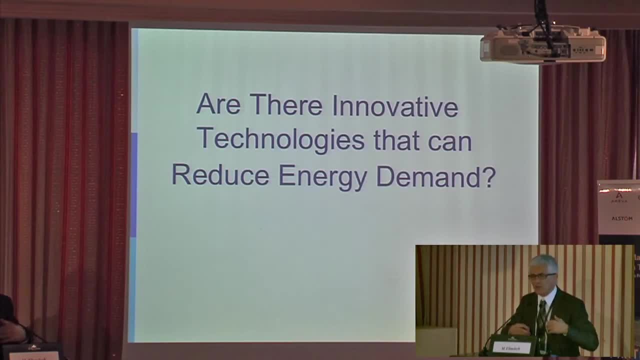 But they were built many, many years ago, And the new plants that are built now, almost all around the world, are reverse osmosis technologies, including the recent one that was built just in Agadir, Morocco. So I would like to highlight the process. 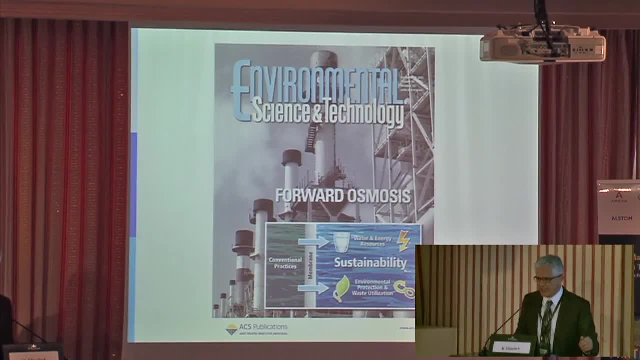 that we are working and conceptualize at Yale University. It's called forward osmosis And see that again, we are not testing it. It may be able to use some energy in desalination, So forward osmosis, the principle. 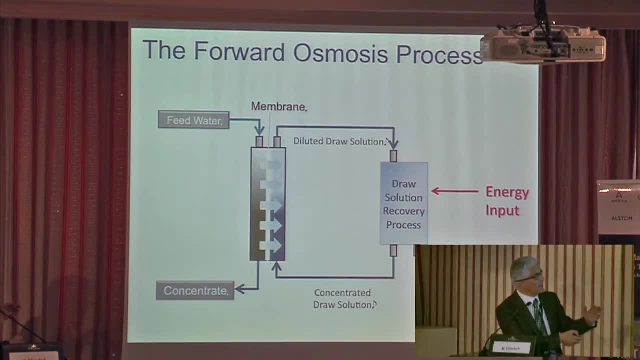 is that you have a membrane here. If one side you can have seawater, if in the other side you will put a solution of higher concentration, then water will move by osmosis to this side. But again, you don't do much here. 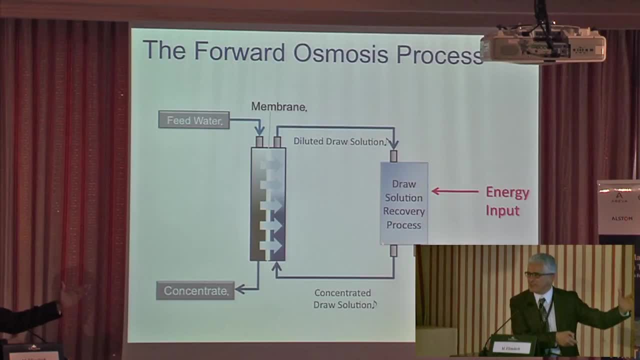 because you take water from the salt water and put in another salty solution, although it's a clean solution, And then if you can find some way to recover the fresh water that passed and reuse the salt solution again, it will be a viable process. 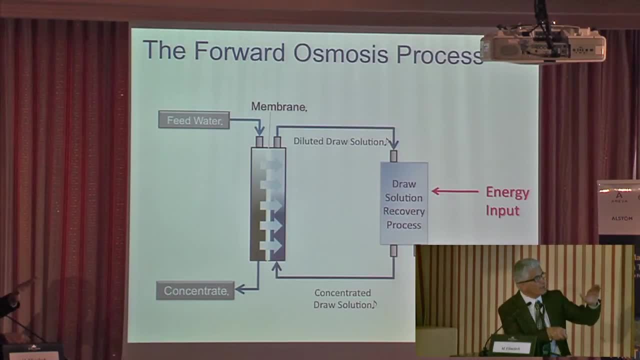 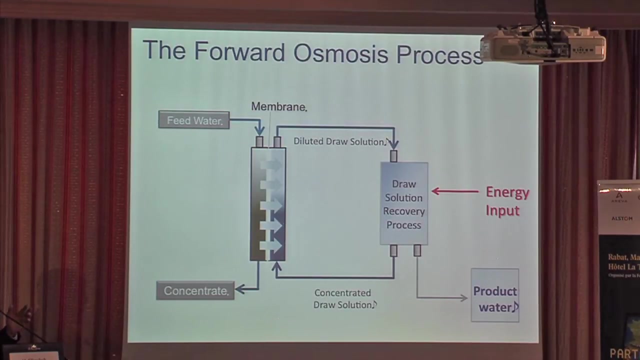 And this is all the energy. All the energy comes here on the process that you recover the clean water that passed through the membrane and reuse this high concentration salt again. So now we need to come up with some nice or some clever solution for this salt. 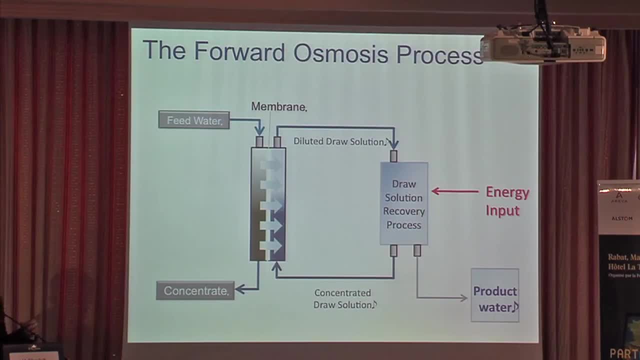 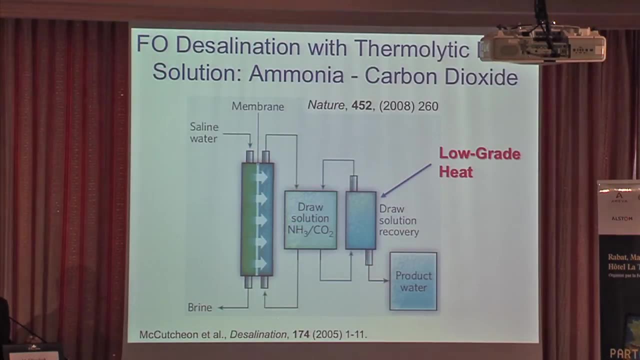 Otherwise, if you need to use another reverse osmosis to separate here, you will not save energy. So we came up with something that we call thermolytic draw solution. Thermolytic draw solution: these are solutions that if you apply some heat, you can decompose them. 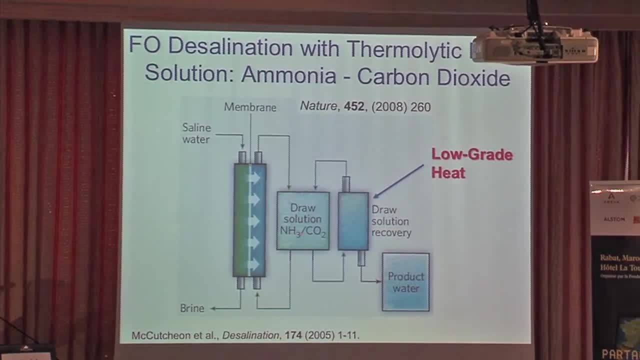 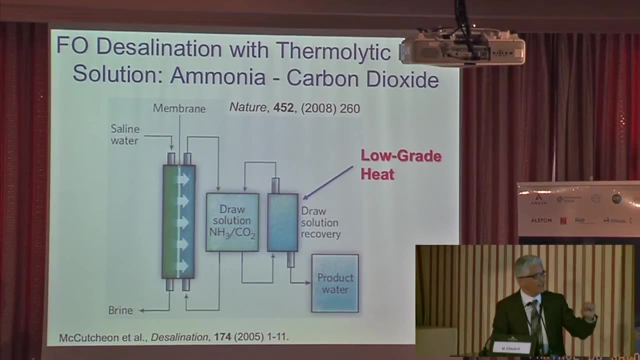 to something. For example, our solution: we have ammonium CO2.. And I will soon show you how it works. I have some animation. Hopefully it will not be affected by the conversion to Mac And this draw solution will draw water. 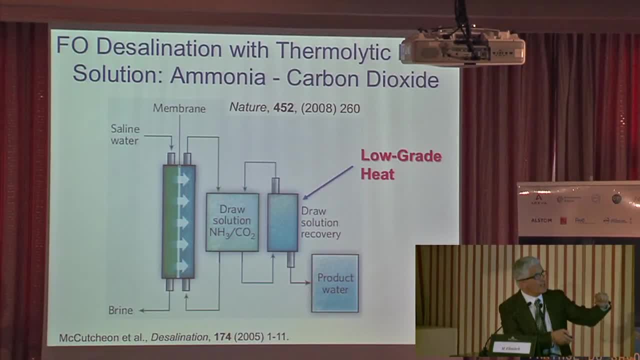 from the foot. So this is a very good solution for the osmosis side And you will need low-grade heat. If you have an atmospheric pressure 58 degrees Celsius, you'll be able to break the solution again and use them and get the fresh water. So let's see how it works. As I said, so you apply. if you dissolve ammonium CO2, you will get ammonium salt. Three types of ammonium salt. First, you apply osmotic pressure So this can draw water across the membrane. 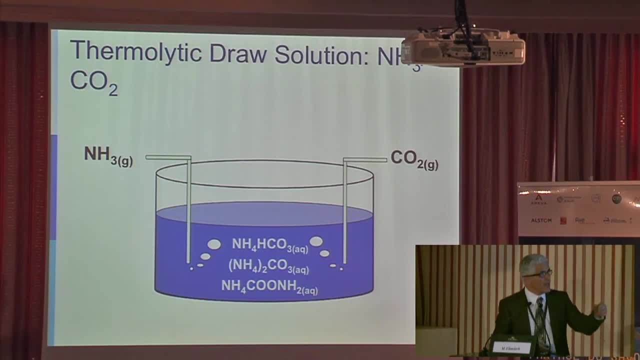 because it has higher osmotic pressure than the seawater. And then, as I indicated, if you apply some heat, you apply low-grade heat or waste heat that otherwise you cannot use it. you can decompose again them to ammonium, CO2,. 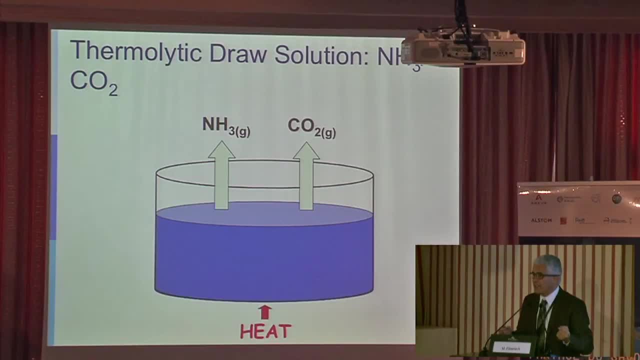 use them again and stay with the fresh water. Now, if you calculate the energy here, it will be much, much more than reverse osmosis, because you know that thermal processes are not as efficient. However, the cost will be insignificant because if you use 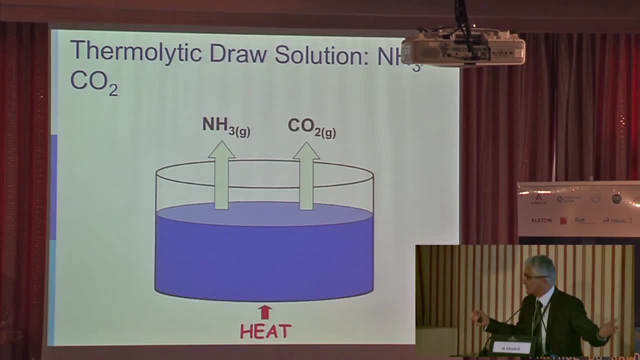 waste heat that otherwise you cannot do anything with it, then it doesn't cost a lot And the electricity that you need here just for the pumps will be maybe about 0.5 kilowatt hour per cubic meter at most. So much, much less electricity as long. 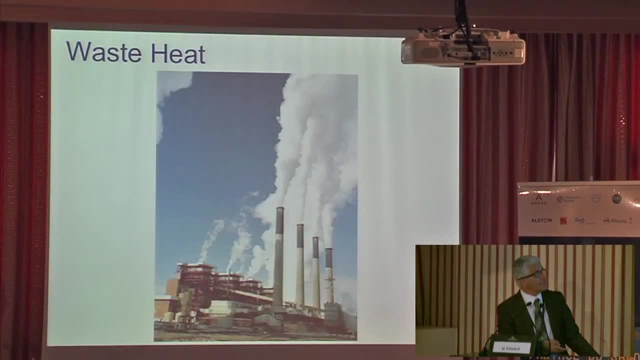 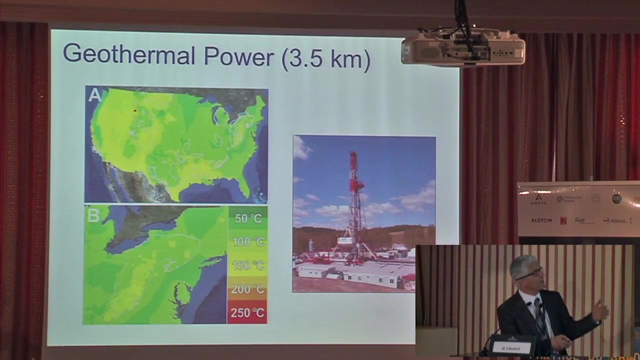 as you have this waste heat. So this waste heat can come either from a power plant or any industrial plant that otherwise will be discharged to the environment. You can also have geothermal energy, So if you have a geothermal- indeed, this is just a map. 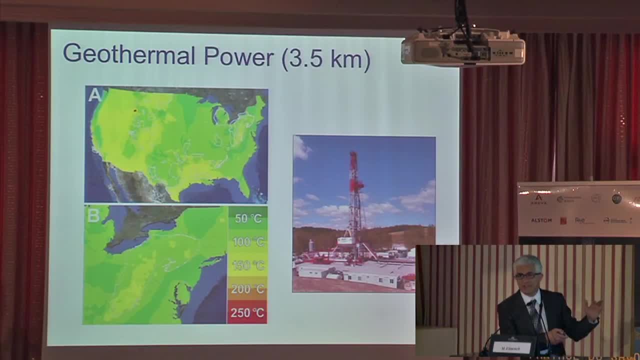 I use it for another paper that we are writing. But if you drill a 3.5 kilometer, this will be the thermal, the temperature that you can get there. It's about most of the United States, about 50 to 100 degrees. 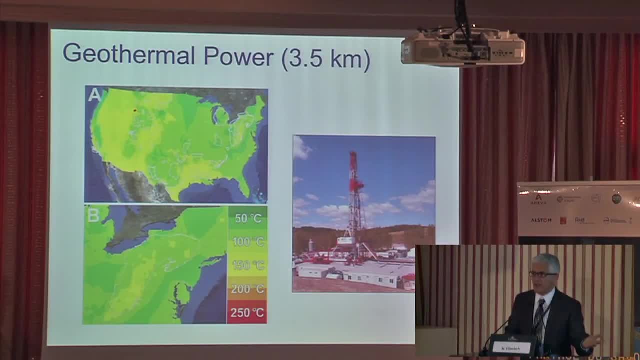 which is good enough for this process, And some places here in the Western United States you can get much higher. Now the reason- if you- those of you familiar from the US- you see this is the area of Pennsylvania And this area is a very, very high salinity area. 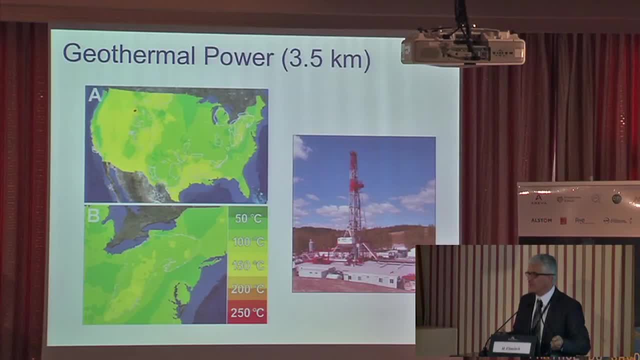 And this idea of the forward osmosis. now there is a company who commercializes it and try it on this water that come from shale gas production. When you produce the shale gas water you get a waste of very high salinity. It can be five times more than seawater. 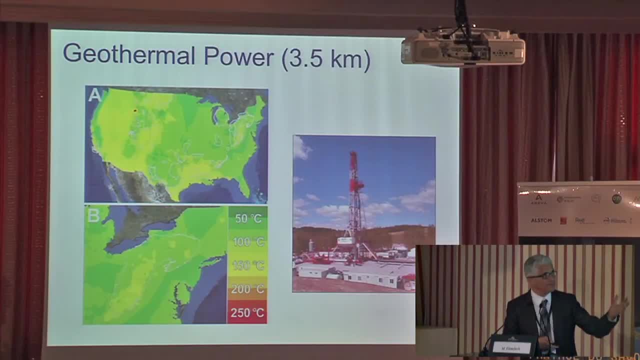 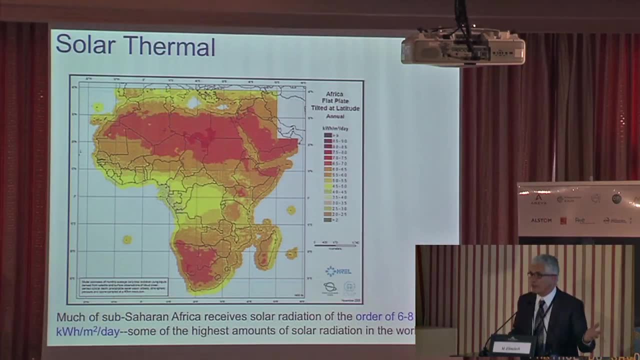 And you cannot treat it by reverse osmosis. The only way you can treat it by this kind of process is the need thermal energy, Or you can use just solar thermal, And we had an excellent talk here from Total Energy, which is a very, very good company. 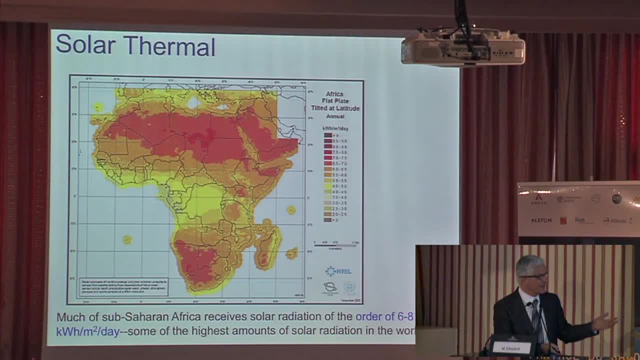 Again, this is just in sub-Saharan Africa. I mean it's plenty. The average there is in the order of 6 to 8 kilowatt hour per meter square per day And in principle you can think about this kind of reverse osmosis. sorry forward osmosis unit. 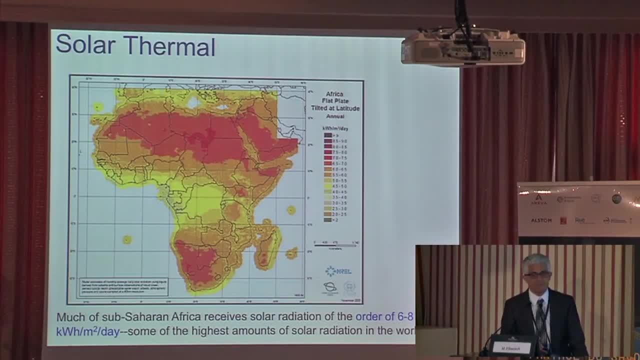 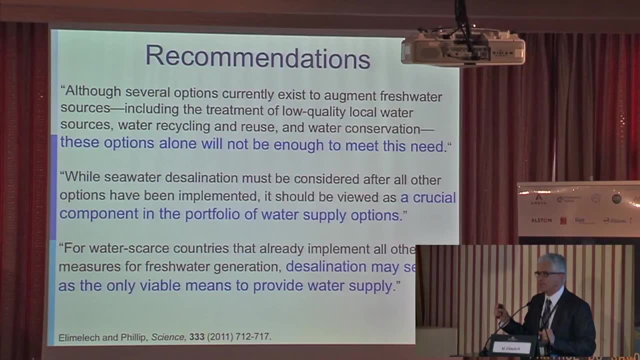 more like decentralized and small unit that can supply water just by using thermal energy. So, anyway, so I would like now to conclude with some recommendations, And these I took directly from the science review article that I wrote in the last two years, And these recommendations were mainly: 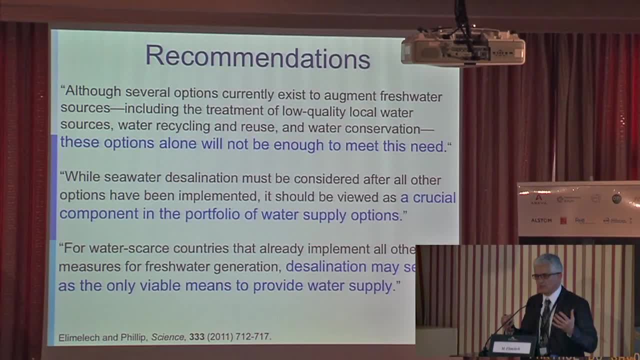 when we were invited to write this article by science, they wanted us also to say: OK, is it really a sustainable solution, Or do you really recommend desalination as a way to solve our global water scarcity? So these are the recommendations that we 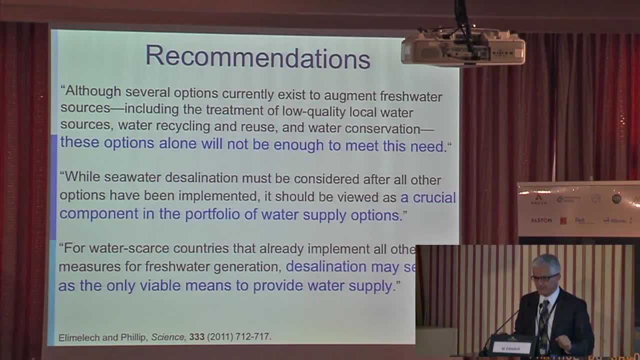 have made at the end of this relatively scientific article, And I'm quoting them directly. So the first one: although several options currently exist to augment freshwater sources, including Including the treatment of low-quality local water, water recycling and water conservation, 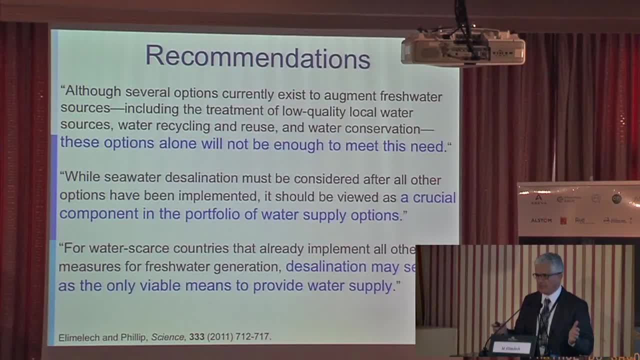 these options alone will not be enough to meet the need. So you can do all the things, but you still need water in many, many places, including North Africa and California and the Middle East and so on, Because some environmentalists in the US- they said no way. It's more like a resistance to nuclear or hydrofracking. No way. desalination, It's too much energy intensity, It's too expensive And you will contaminate the ocean and everyone will die, and so on. Now, while seawater desalination must be considered, 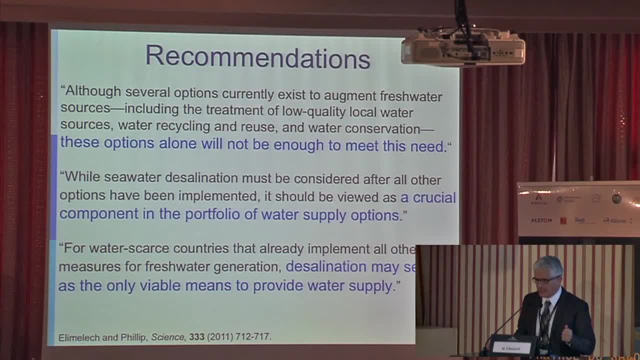 after all other options have been implemented, it should be viewed as a crucial component in the portfolio of water supply options. You need to try all the other options, because this one is three to four times more energy, But if you've done them and you have no water, 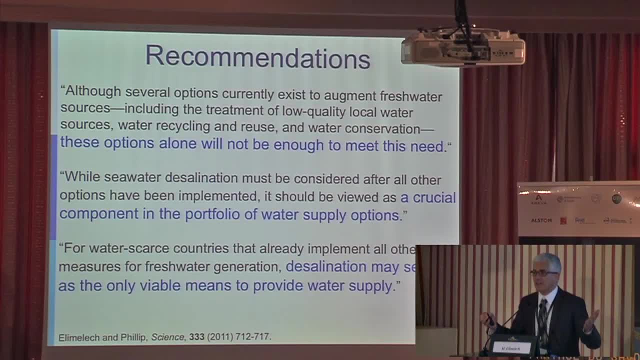 this should be part of the portfolio for water supply, Because water supply is like energy: You have a portfolio of water supply and you cannot say that all the water comes from one source. You can have some water that comes from rivers, some groundwater, some desalination. 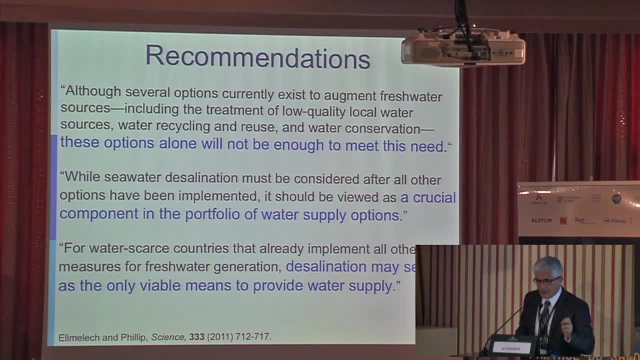 some recycled wastewater and so on. And lastly, for water-scarce countries that already implement all other measures for freshwater generation, desalination may serve as the only viable means to provide water supply. So we really here recommend, and again, although many scientists 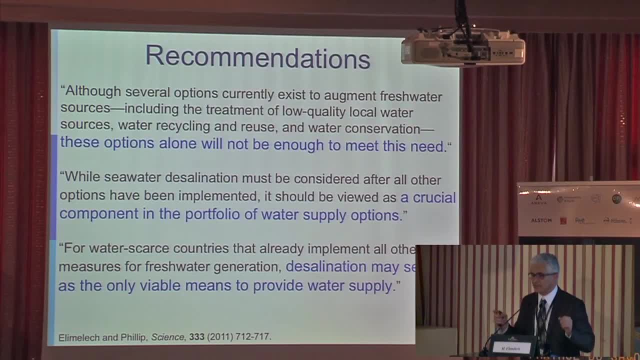 and environmentalists object, at least in the United States and some of the Western countries, that if you try all the options, this is a good way And although it's energy intensive, it's not unusually energy intensive and it can be used part of the energy portfolio. 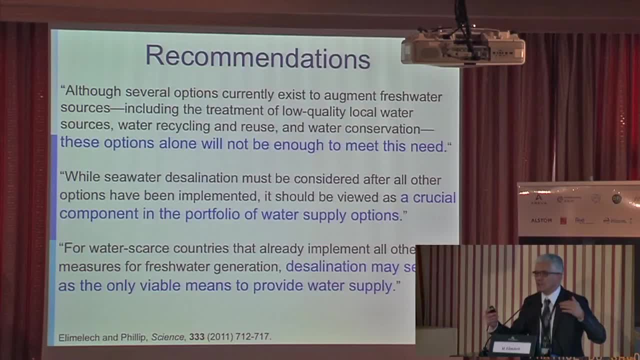 Now here I talk mostly with application to the developed world. Again, if it's applied completely to the developing country, probably not, But anything in between it's suitable. And indeed you hear many countries now that build desalination plant: Algeria. 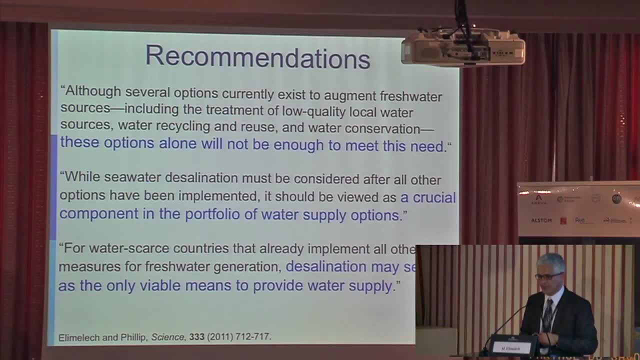 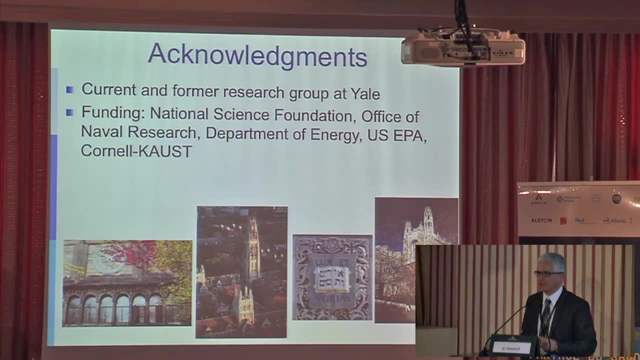 Morocco, China and so on, So it's become really a global solution. So I would like just to thank the former students that did all the work and the funding, And these are some pictures from Yale University. Thank you very much.